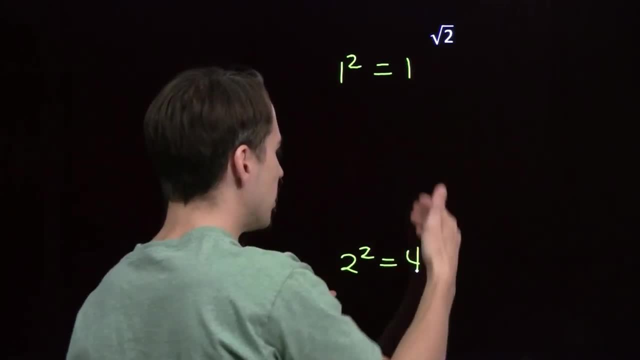 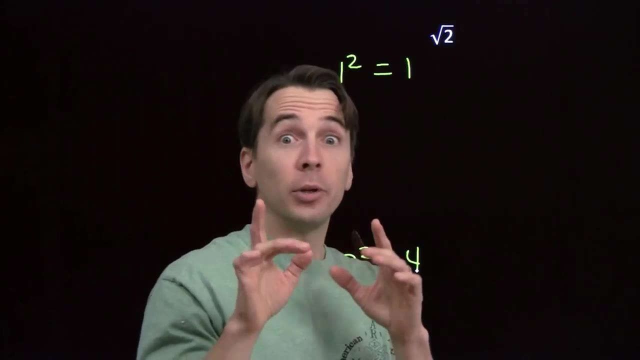 is 16.. That's no good. So square root of 2 has to be between 1 and 2.. But there aren't any integers between 1 and 2.. There are numbers between 1 and 2.. Try 1.5.. 1.5 squared, that's. 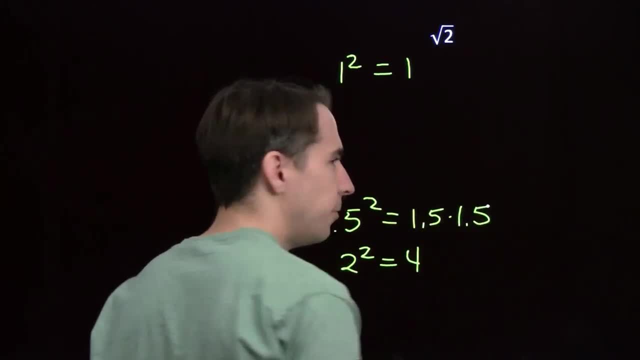 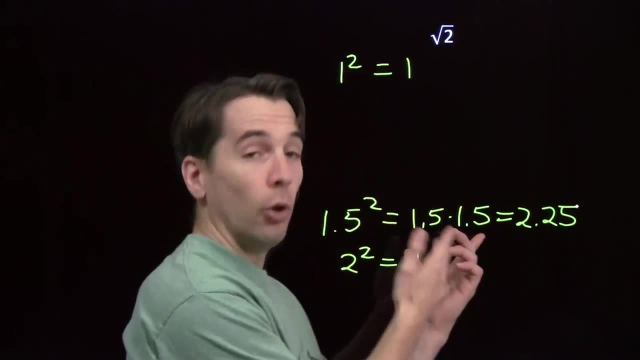 1.5 times 1.5.. 15 times 15 is 225.. So 1.5 squared that's 2 point 2, 5.. It's closer to 2, but it's still. that's too high. That's too high. So the square root. 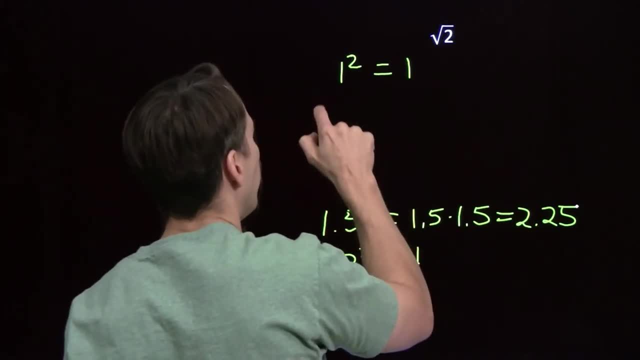 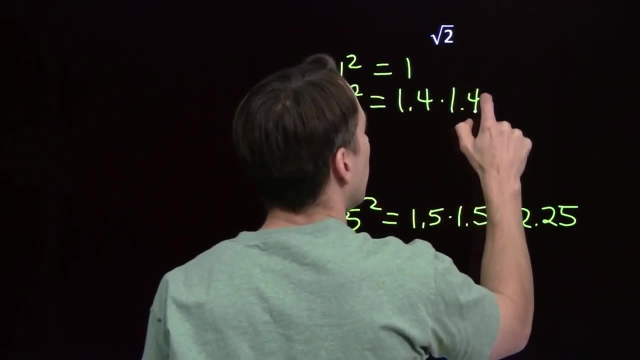 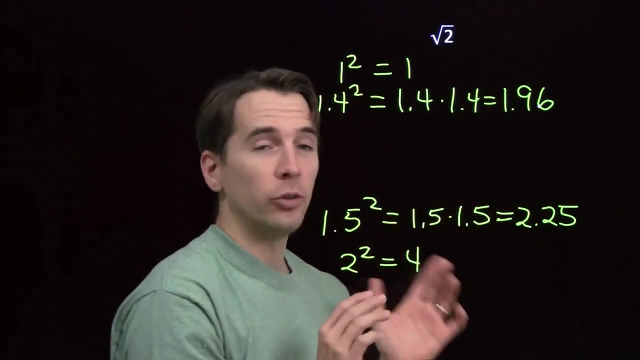 of 2 has got to be less than 1.5.. Well, try 1.4.. 1.4 squared is 1.4 times 1.4.. 14 squared is 196.. 1.4 squared is 1.96.. It's closer to 2.. It's closer to 2, but it's less than 2.. 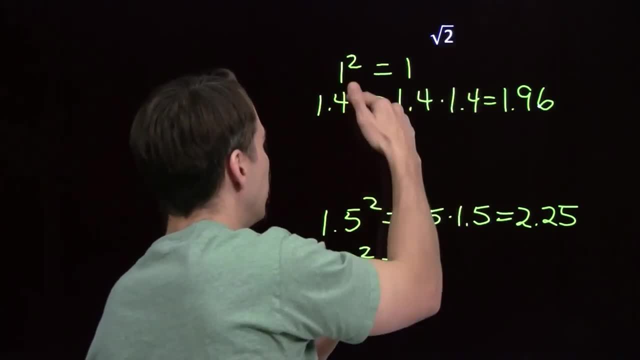 So this: this isn't large enough. So the square root of 2 has got to be between 2 and 1.5, squared 1.4 and 1.5, which means we need more decimal places And we could keep. 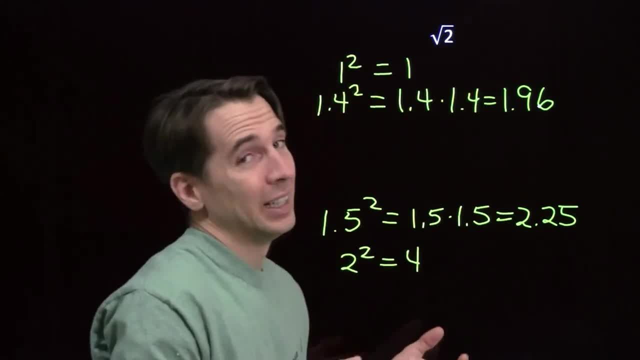 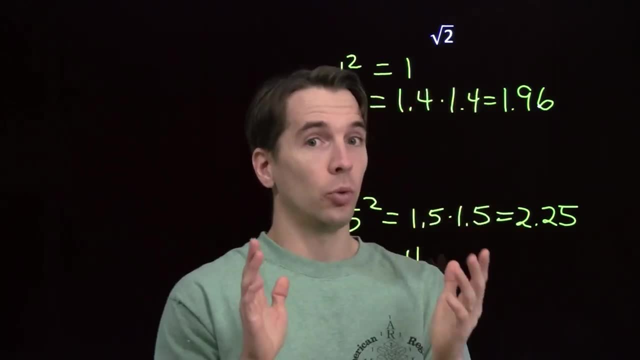 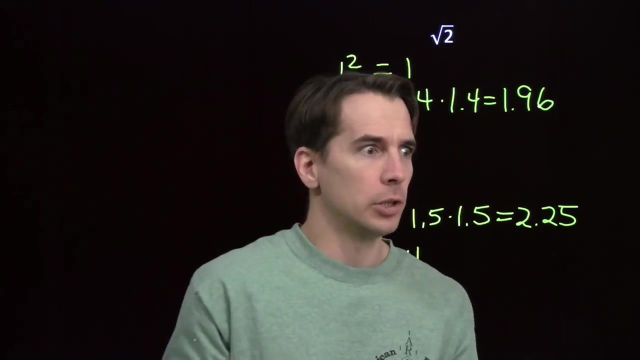 going on like this, but I mean it might take forever And in fact it turns out that it will take forever. This is a very special number- Square root of 2, we can't write it as a nice neat terminating decimal. We can't write it as a repeating decimal either. 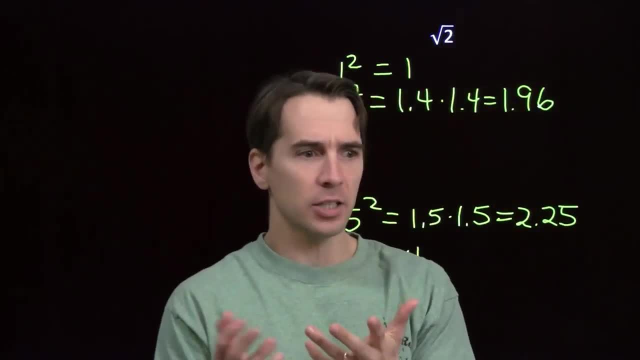 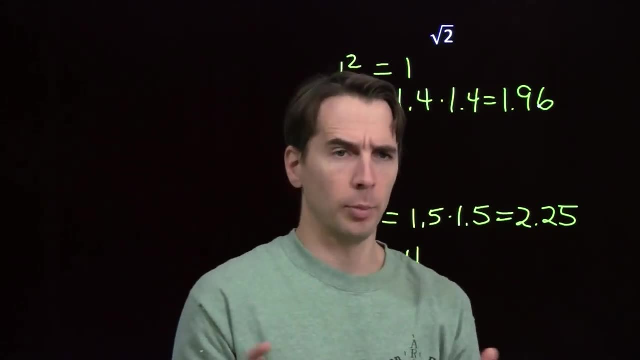 So you might think: hey, let's try fractions. But we can take any fraction and write it as a repeating decimal Or a terminating decimal. You know, if you start with one integer and divide it by another, you're going to get a terminating decimal or a repeating decimal. So I can't write the. 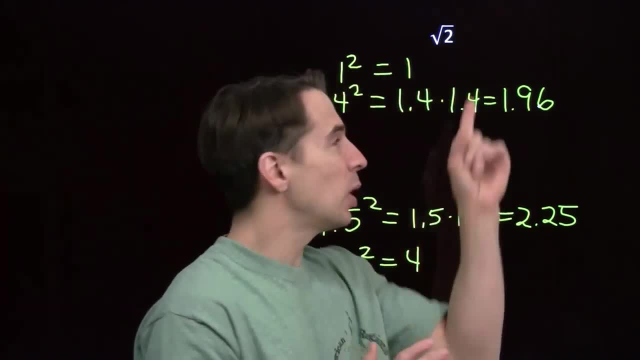 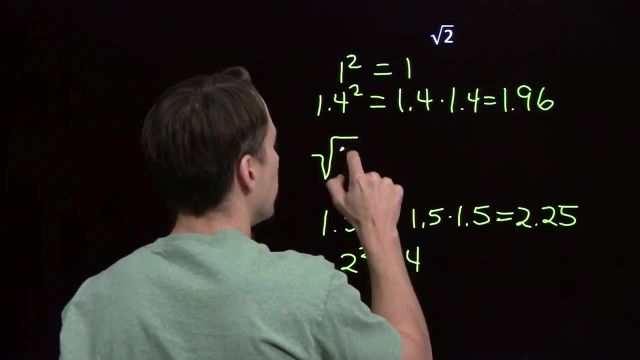 square root of 2 as a fraction, either. It's a very special number and this is the best way to write it: The square root of 2, that's the best way to write it, and that's the number that we square to get 2.. I mean, that's just the definition of the square root, The square. 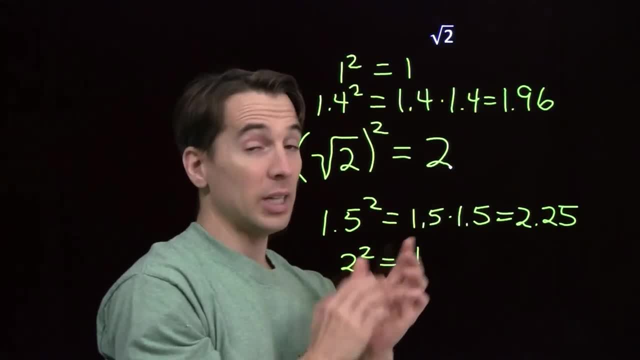 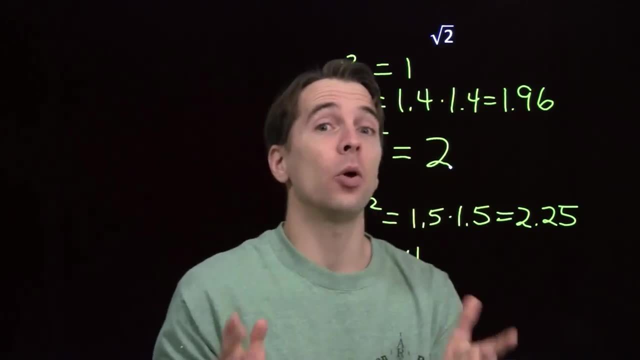 root of 2 is the number we square to get 2.. And this is the best way we can write it. We can estimate it. We can estimate it with decimals or fractions, but we can't hit it exactly. It's a very weird number, It's so. 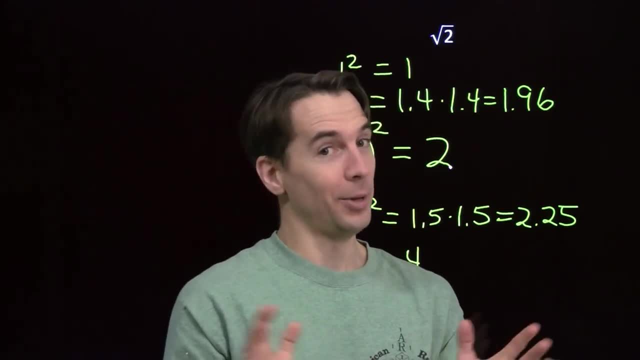 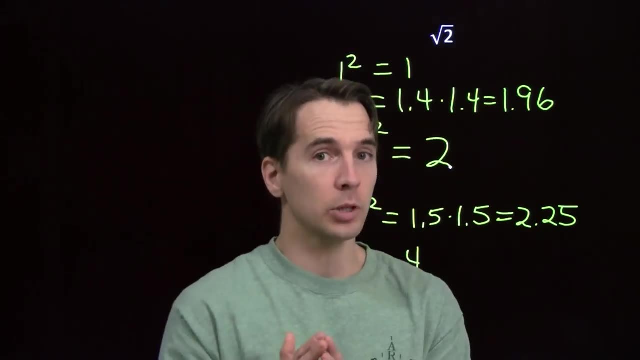 weird that mathematicians call it irrational. I'm not kidding. This is what's called an irrational number. You can take a number and write it as one integer divided by another, like the fractions we've worked with. Those are called rational numbers, This number. 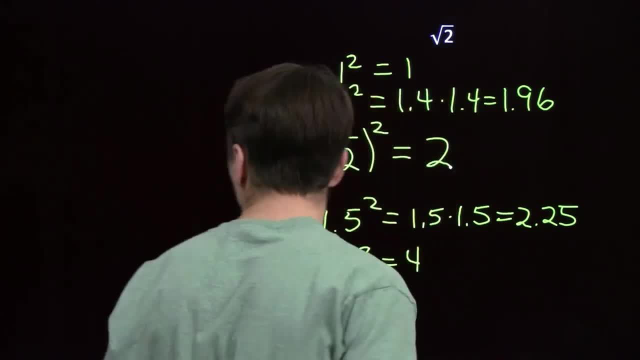 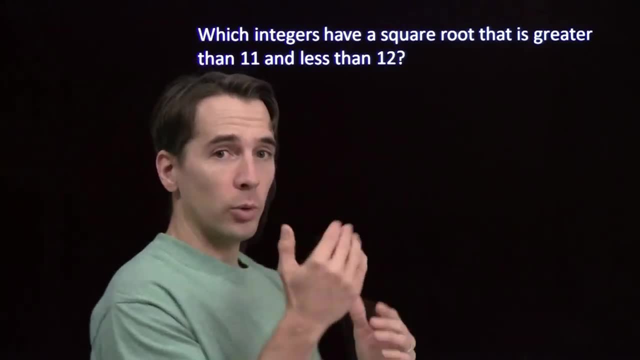 we can't do that, so we call it irrational. Let's look at a few more problems involving these irrational numbers. We'll start with this one. We've just seen a number that has a square root between 1 and 2.. Let's look for the ones that have a square. 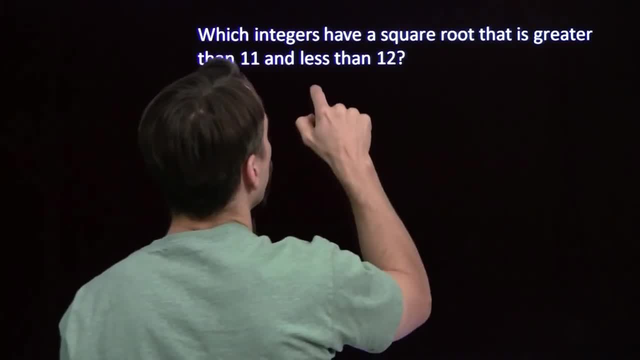 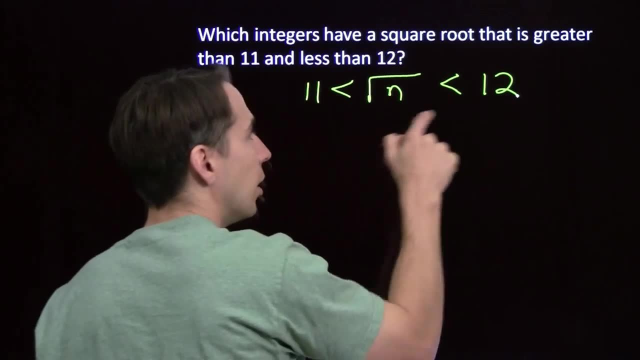 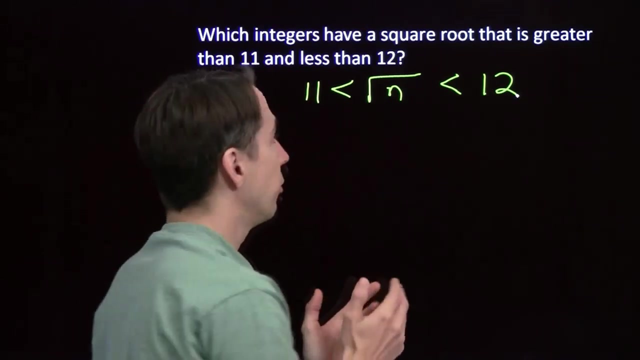 root between 11 and 12.. What we're looking for here are the numbers, the integers, whose square roots are between 11 and 12.. Now, of course, the square root can't be an integer, because there aren't any integers between 11 and 12, but if the square root of n is, 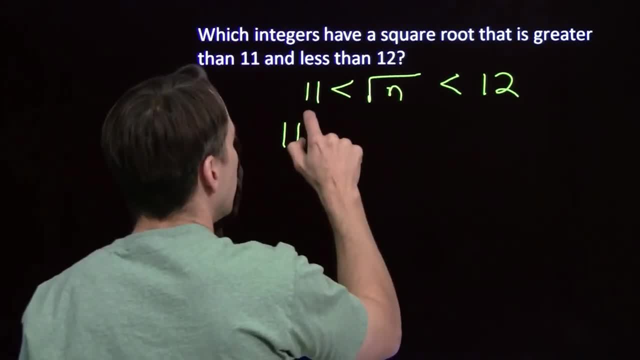 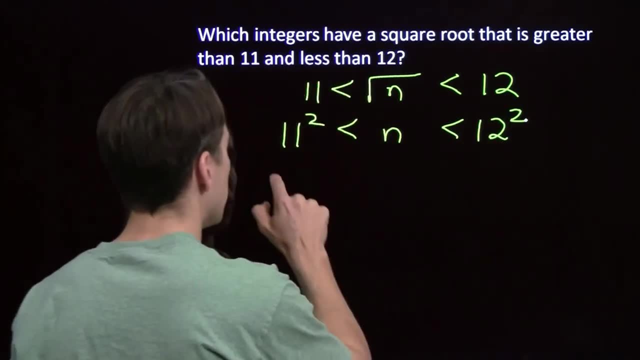 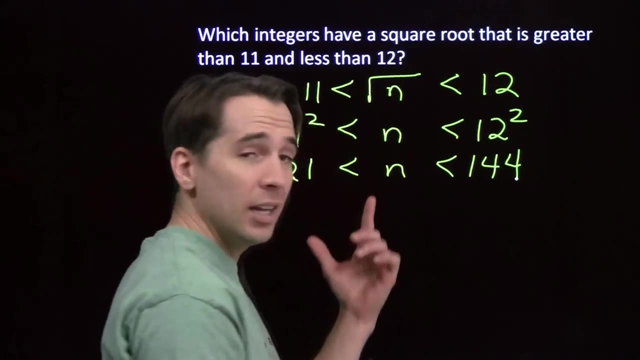 between 11 and 12,. that means that n has to be between 11 and 12.. If that's true, then 11 squared and 12 squared, Of course. 11 squared, that's 121, and 12 squared is 144.. So n could. 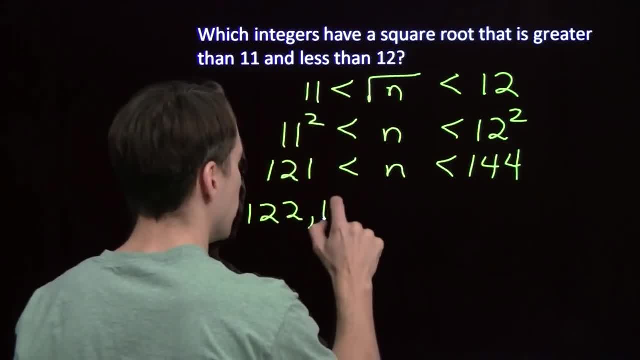 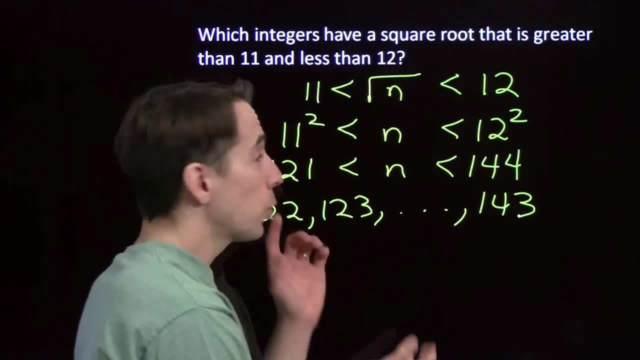 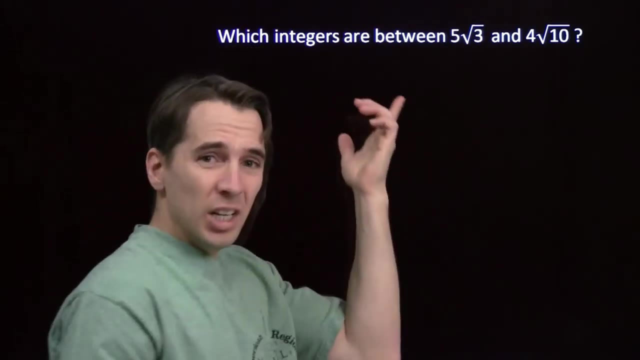 be any of the integers 122,, 123, and so on up to 143.. And these are the integers that have square roots between 11 and 12.. Let's try another one. Which integers are between 5 root 3 and 4 root 10?? Now it's not at all obvious to me what integers you know even. 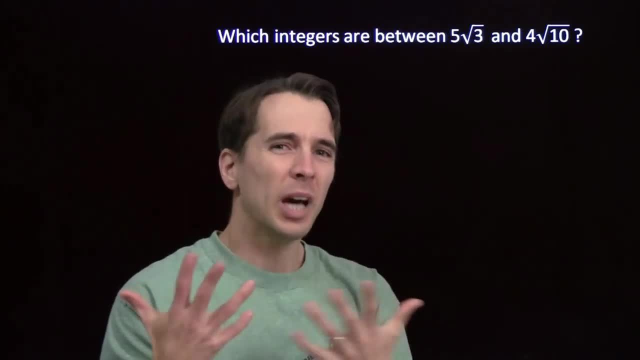 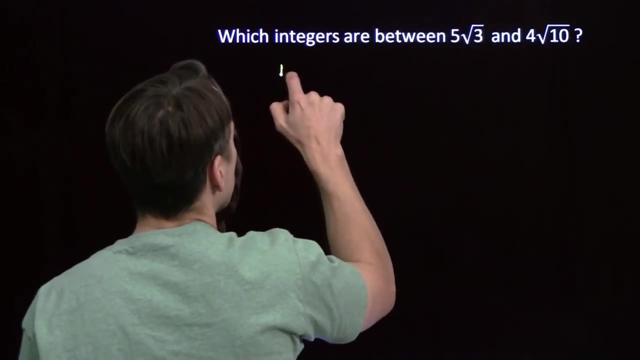 5 root 3 are near and what integers are around 5 root 3, but we've got to feel for the square root of 2 by looking at squares. Let's try the same thing here, because we do know how to square that number. I can take 5 times the square root of 3, and I can square that. 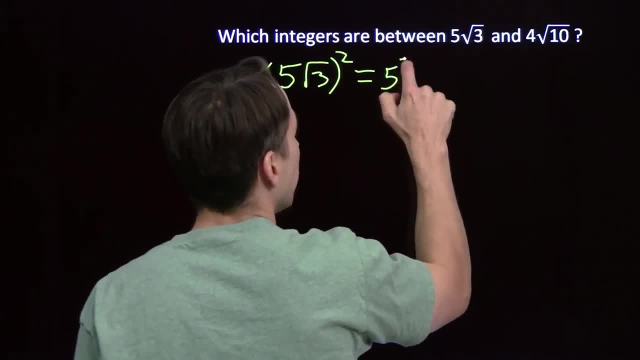 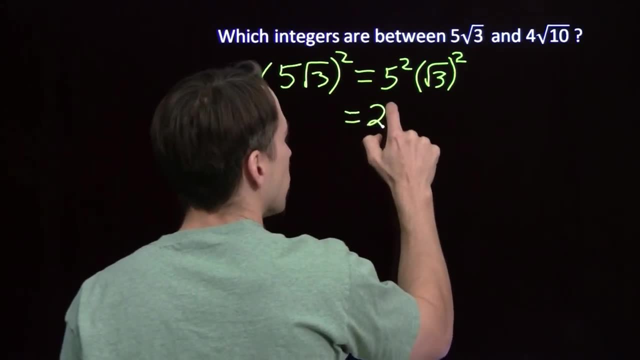 using a handy exponent rule. We just square the 5, and we square that square root of 3, because we know how to square both of these. 5 squared is 25, and when we square the square root of 3,, of course that gives. 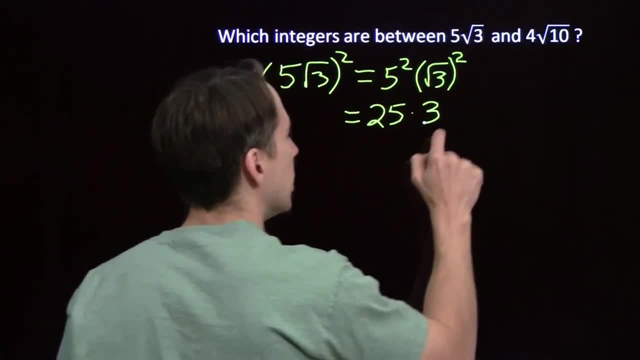 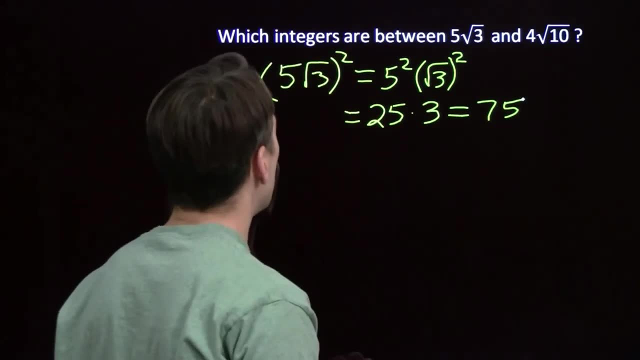 us 3, because the square root of 3 is the number you square to get 3.. So that gives us 75. So we know that the square of 5 times the square root of 3 is 75. So 5 times the.